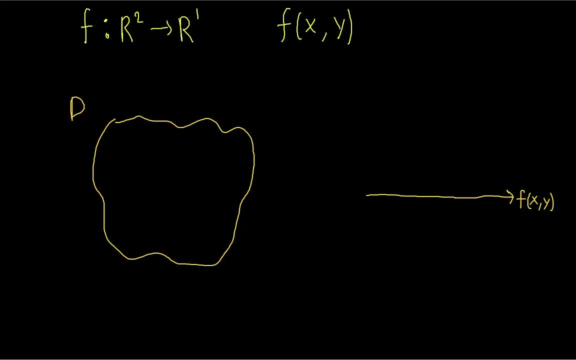 domain is now two-dimensional, So the input, instead of approaching a single x value, it's going to be approaching a point on this domain. So, again, if we can make the value of the function as close as we want to this number L by restricting the input values, 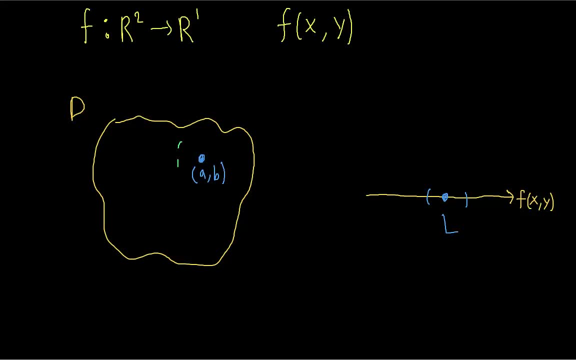 to some interval around this point A- B. then we say that the limit as x, y approaches A B of the function is equal to L. Notice that now, since our domain is two-dimensional, instead of just an interval around some point. 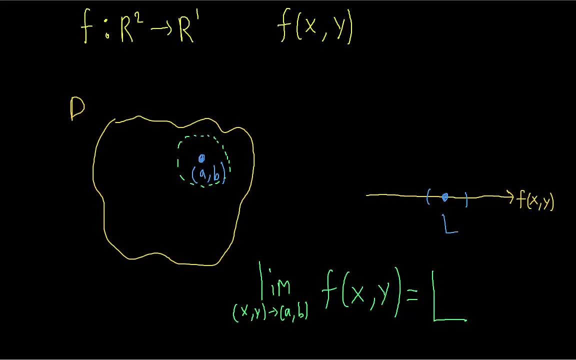 we have a disk around the point. So if this limit exists, then we must be able to make some disk around the point A, B, such that for all of the values of x and y inside this disk the value of the function is very close to L. So you can see that it's basically the 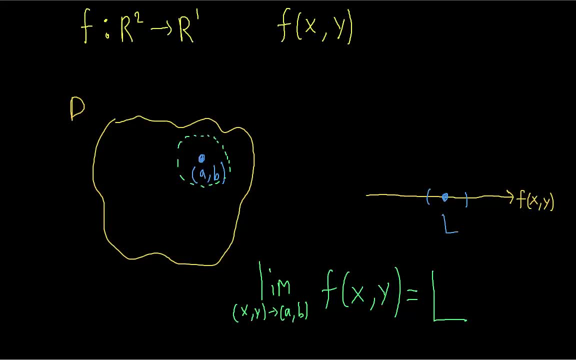 same idea. So in this video we're not going to go over the formal definition of a limit. We're going to look at how to prove that a limit does not exist. So the key thing with multivariable limits is that as we approach this point A, B in 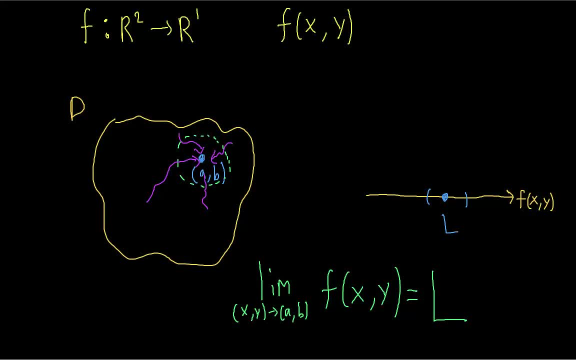 the domain, the function must always approach the value L, No matter how or what path we use to approach A B. So oftentimes when we're evaluating limits then we choose a specific path to approach the point A B on, because it's easy to calculate it that way. 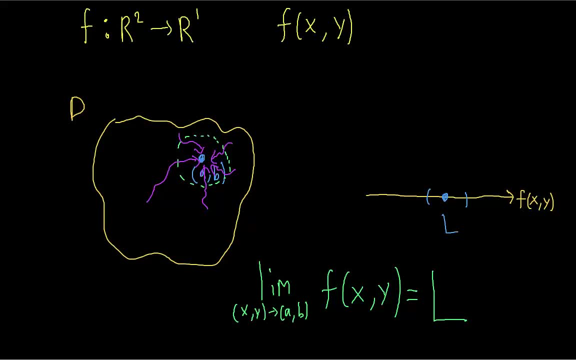 So no matter what path we take to approach this point A B, the value of the function has to approach the same value. So this is similar to how in single-variable limits, the right-hand limit and the left-hand limit have the same value. So this is similar to. how in single-variable limits, the right-hand limit and the left-hand limit have the same value. So this is similar to how, in single-variable limits, the right-hand limit and the left-hand limit have the same value. So this is similar to how, in single-variable limits, the right-hand